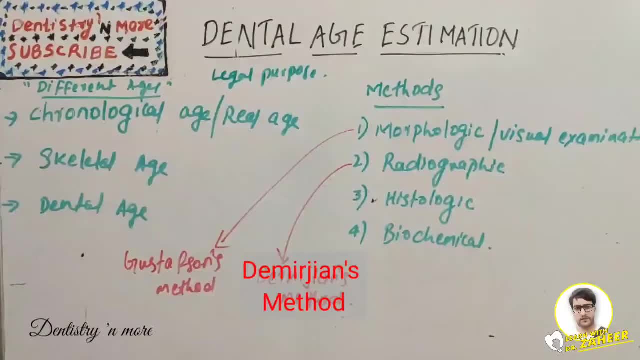 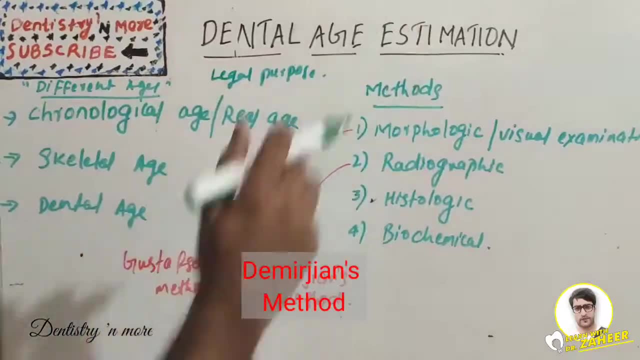 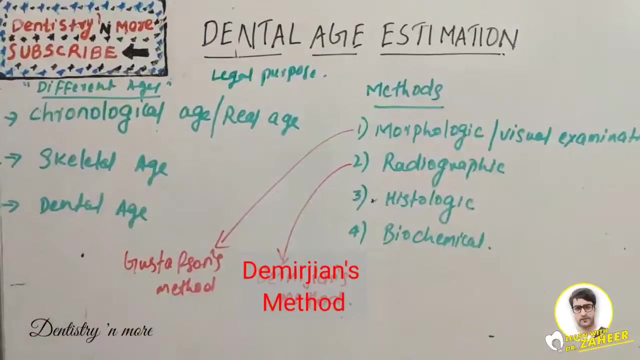 So you just cannot skip this chapter for on exam point of view. So mostly asked questions are the dental age estimation, then the histologic method of dental age estimation- Gustafsson's or Demerjian's method. So let's see one by one. This will be dealt in a few sessions. Today's session is about the two methods, that is, the morphological method Gustafsson, and the radiologic method, Demerjian's. 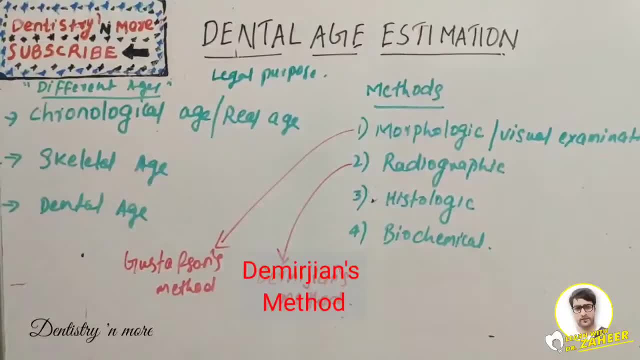 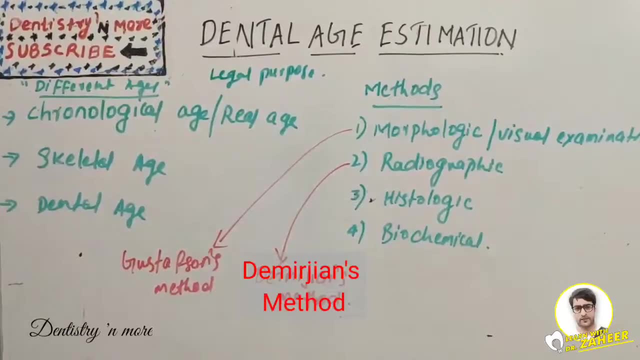 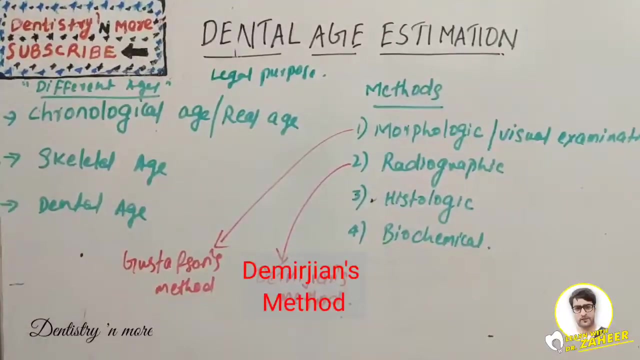 So we'll start with some basic idea of dental age or age estimation. So age estimation is an important factor in biological identification in many forensic fields such as forensic odontology, forensic medicine, forensic anthropology and forensic osteology. So it helps to narrow the search possibilities for unidentified dead people or living individuals, mainly for the legal. 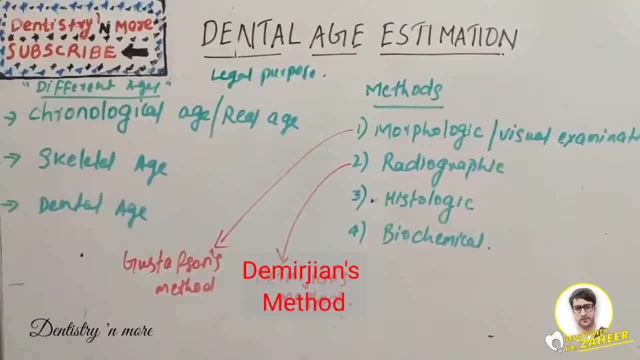 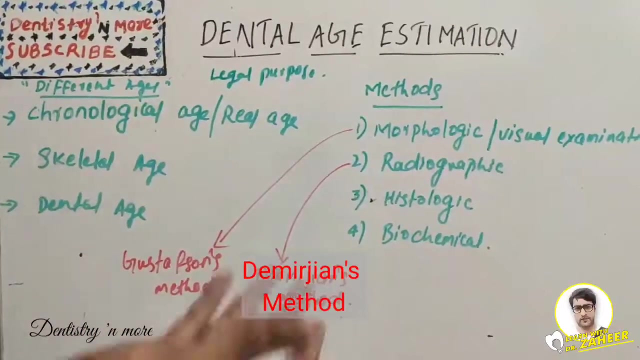 purpose, And it also helps to determine the age of criminals, for mainly those who are in the younger age group, because the age- if they are adult, the punishment they get is different, and if they are minor, the punishment they get is different. So, in order to prove their real age, we can depend on the various methods. 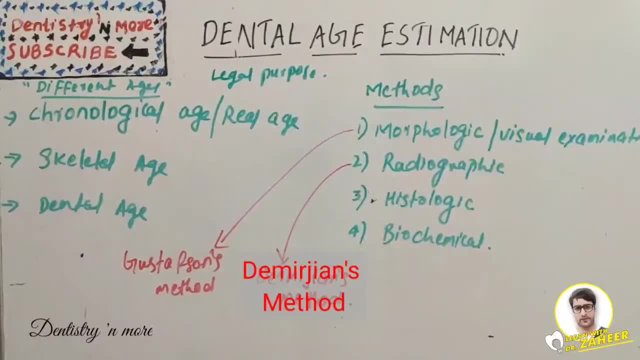 So, therefore, accuracy of age estimation methods for suspects with unknown chronological age who are involved in any type of crime is needed in the interest of justice. So first we need to understand few terminologies, that is, what is chronological or real age, what is skeletal age and what is dental age. 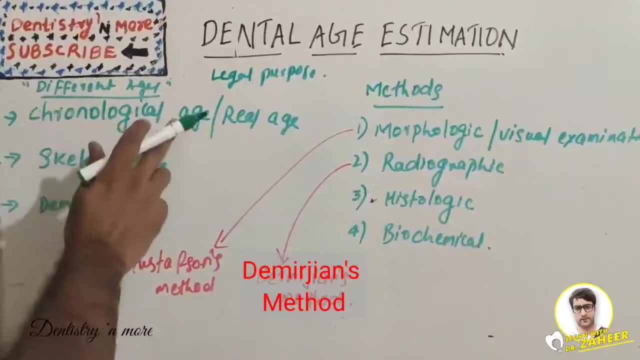 The first one is chronological or real age. The second one is chronological or real age. The fifth one is chronological or real age. The sixth one is chronological or real age, That is, the age in which the criminal is actually talking about, measured by the calendar. sometimes it be a period of intrauterine development or 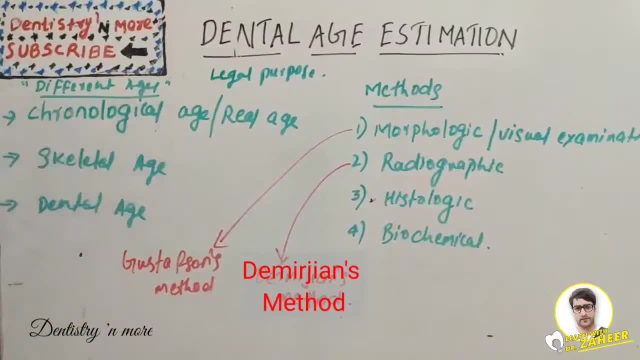 number of years after birth. so this is a commonly known method of age estimation. that is, a chronological age, but as a skeletal age, which is determined by the degree of ossification or development of various bonds which is known to occur at particular time in average individual. so we calculate skeletal age by comparing. 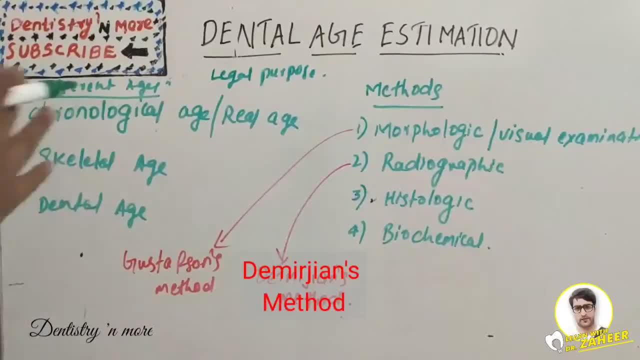 with the ossification or development of various bone. so every bone has a particular pattern of ossification. so we correlate with those bones and calculate the skeletal age. finally, the dental age, which is determined by studying development of various teeth from time of crypt formation- and crypt is when the crypt is visible- till the time of fruit completion. so we have 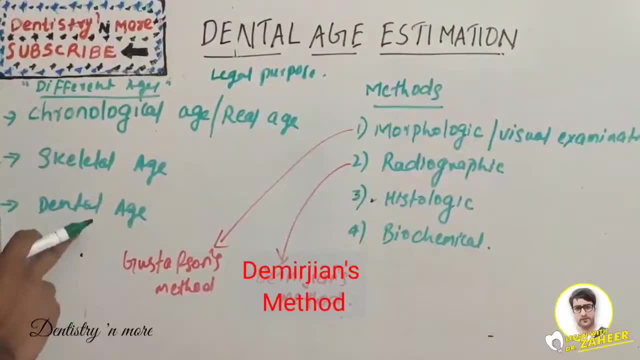 a pattern or a time period where each step of a tooth formation happens for particular tooth, so it it will not vary much in people. so we can correlate those standardized stage of tooth development or a particular tooth and calculate the dental age. so that is what we are going to learn. 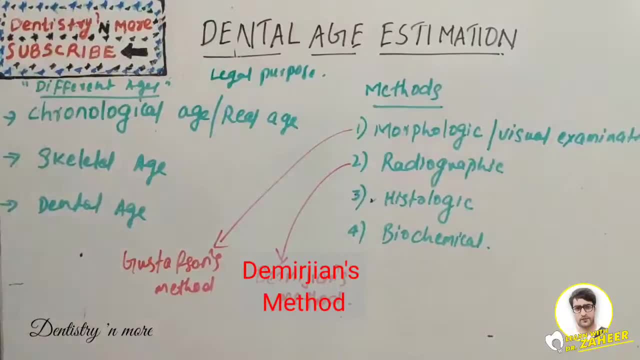 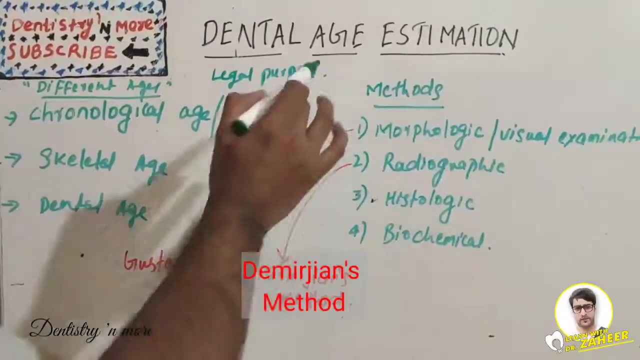 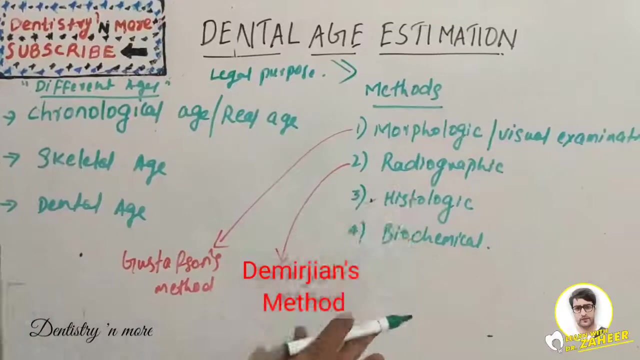 the dental age estimation. so we have lots of method for skeletal age estimation. so today's session is about, for the future sessions are mainly on the dental age estimations. so we have few methods for dental age estimation. they are morphologic or visual examination, radiographic examination. histel X examination and biochemical examination, the morphology, Kong or corporal age or cortical age, and biochemical examination, the morphology Or cic are: visual examination, radiography examination, the stylagic examination and biochemical examination, the morphology or visual examination and radiographic examination and biometpering estimation or part of the output and broad type of file. Sergeant in chin, I believe the examination and biochemical examination results will build up brain, видимossa and so forth And found what we return into thegas, ideally okay. now we can consider fixed adult and have different communities are needed, the different master groups. I think these areas are in the分享 to do what we consider. 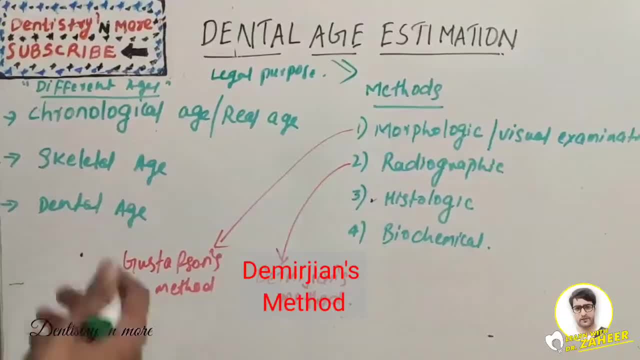 put cameras, The morphologic or visual examination, which are based on the assessment of teeth. that is ex vivo measurement. So ex vivo means in a living person. So these methods require extracted teeth for microscopic preparation. So if a person in a dispute of his age identification, we need to extract the person's tooth. But these methods may not be acceptable due to ethical, religious, cultural or scientific reasons. 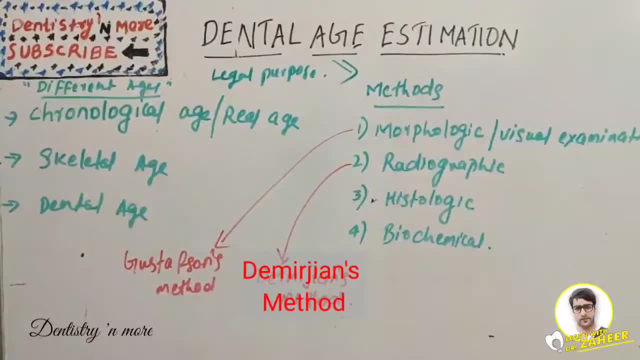 So that is morphologic or visual examination. This is basically ex vivo method. Then in persons, by removing the person that is in a living person. So to extract the tooth we have many problems, So this method is quite difficult. So we have the most commonly used morphological method. 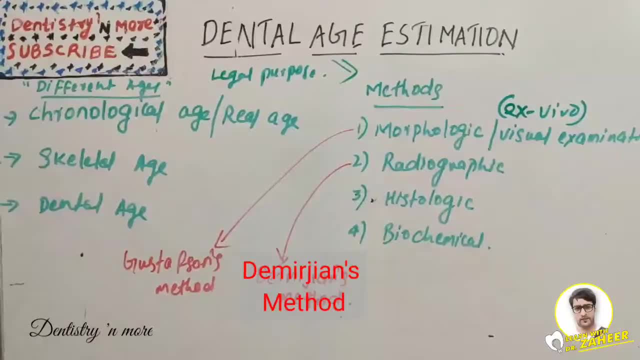 They are Gustafsson method and many methods are there, such as Sohey methods, Maples method, Johansson methods, but the main problem is, which is not possible to be performed in a living person, because we need to take out the tooth and do an ex vivo study that is outside the tooth, with minimal alteration of that specimen. that is, ethically, it's not at all a good thing. 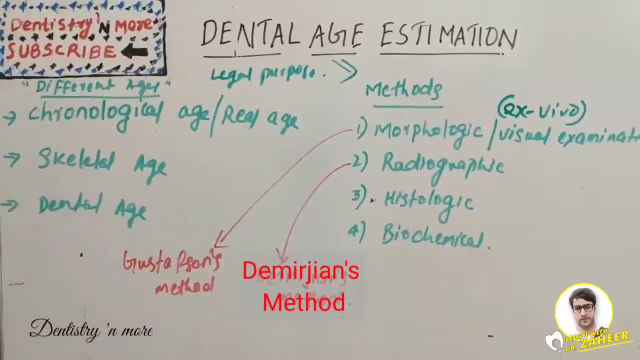 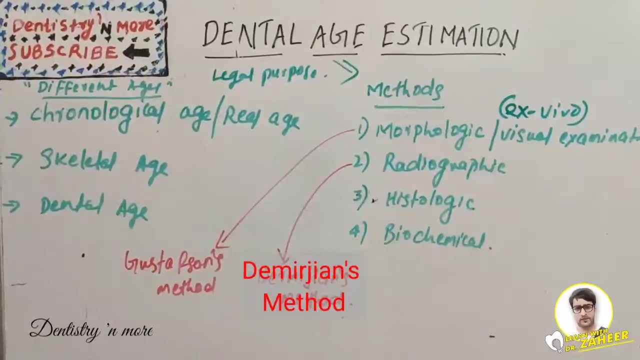 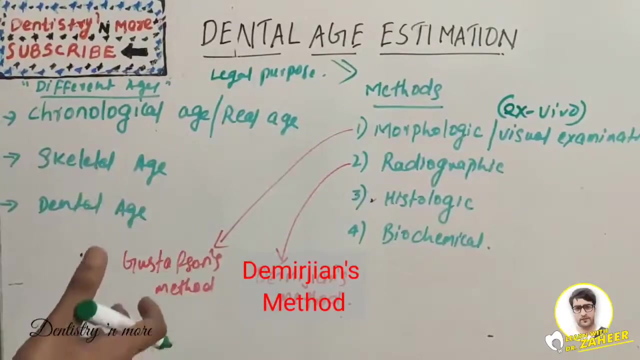 So it is not possible in living person, Whereas the biochemical method, biochemical methods are based on the amino acids, so the amino acid and the rasamization of these amino acids, So the rasamization of amino acid, is a reversible first order reaction and which is relatively rapid in living tissues in which metabolism are slow. 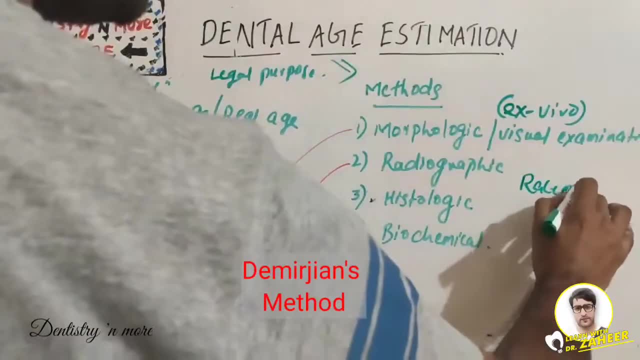 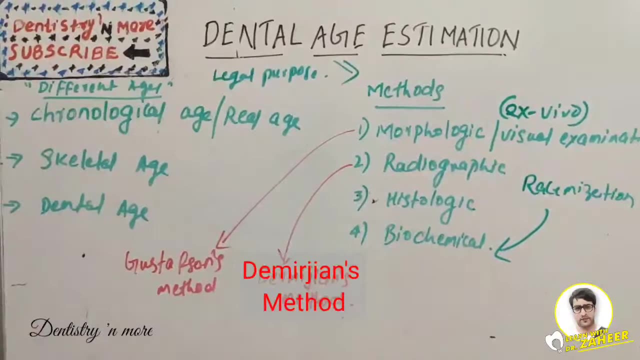 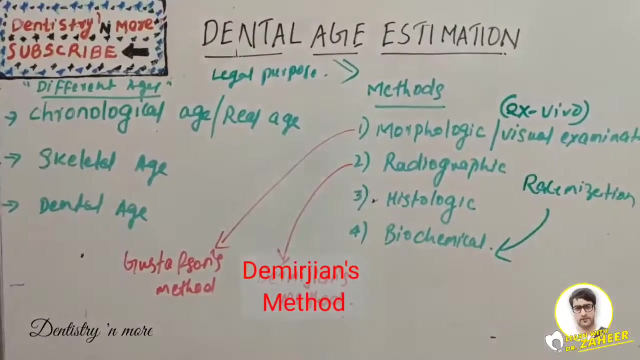 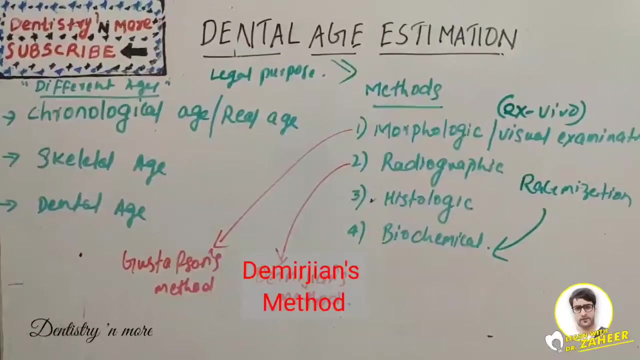 Rasamization So we can correlate with the rasamization process of these amino acids. So the aspartic acid has been reported to have highest rasamization rate of all amino acids and to be stored during aging, So which can be correlated and age can be calculated. 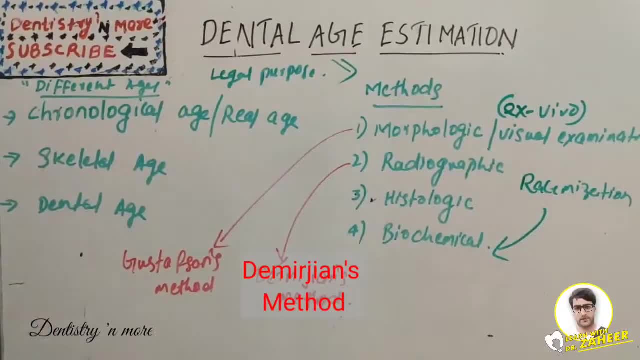 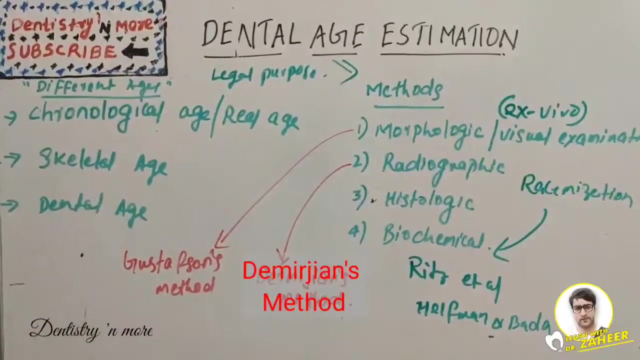 That is the biochemical method. So the Ritz et al method, Ritz et al method and the health man and health man and all are under biochemical methods, Whereas the radiographic method, This follows the pattern of maturation of teeth. So we know teeth having the growth from its creep to the root formation. 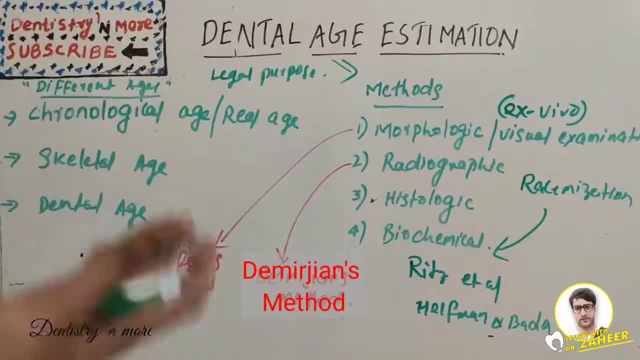 It starts from birth and even it starts in the uterus for the deciduous teeth and starts from birth for the permanent teeth, Which has it starting the first permanent molars during the birth and around seven, eight years and it goes on for the second molars. 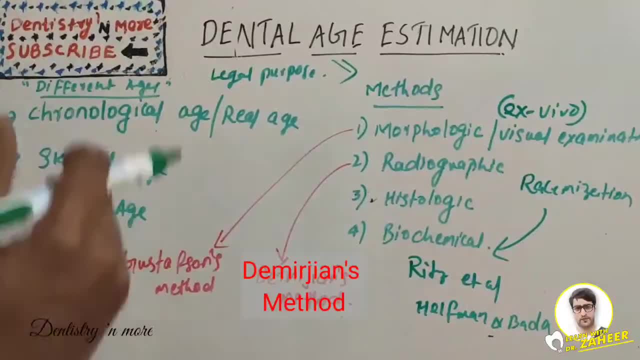 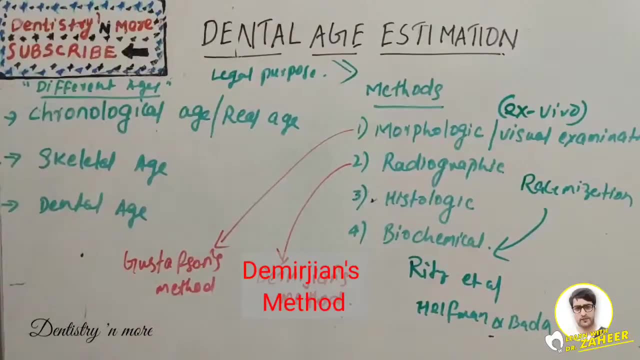 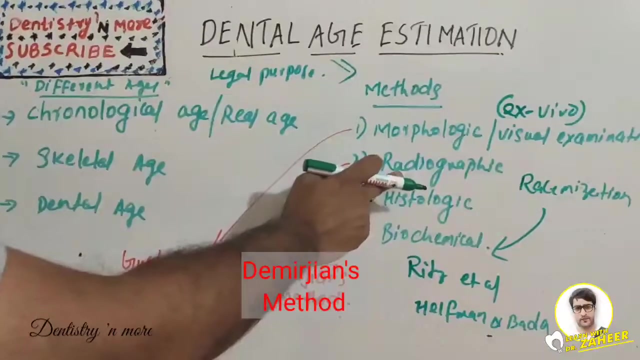 So we can correlate various stages of calcification: The root formation, root completion, crown formation and the layers of crown formation, dentin, enamel, All those can be calculated or do a radiographic examination and correlate with the standard tables. So such method is known as the radiographic method. 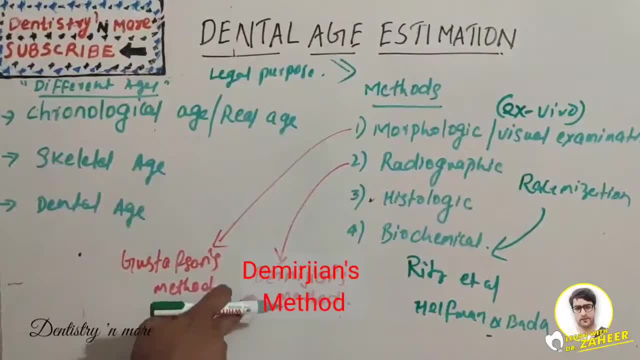 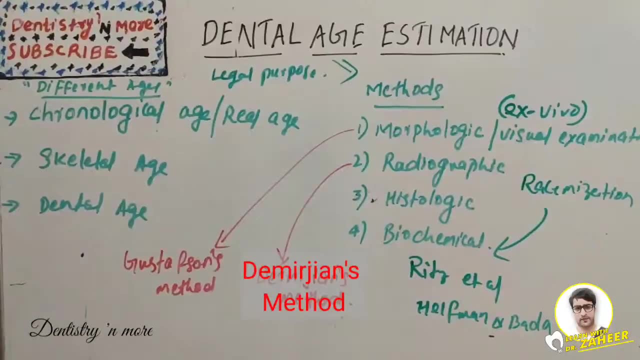 The most commonly used is the dermogeans method. So dermogean has formulated a table for boys and girls And he classified eight stages. where can correlate the formation step or the stage of its formation and convert the stage into a score? 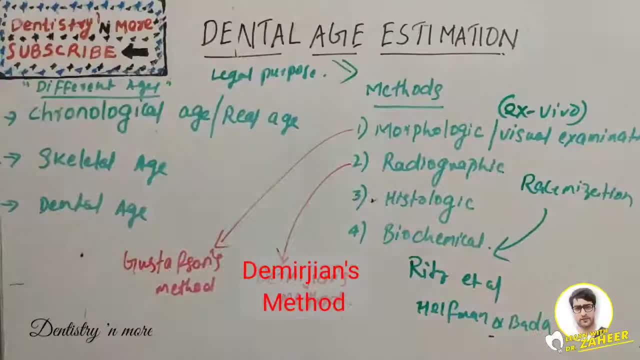 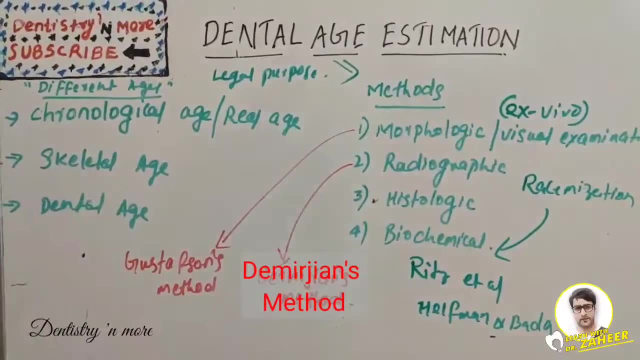 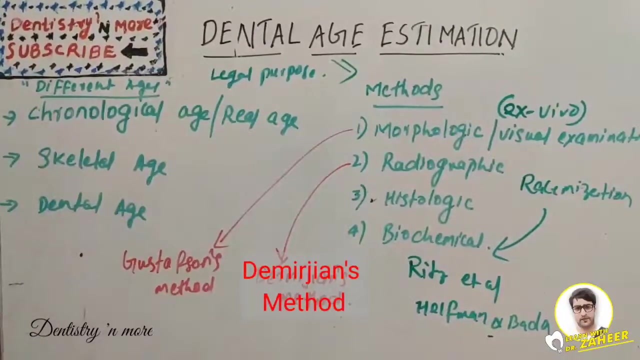 Add all the teeth, score and make the age estimation. So we'll be dealing these two methods in detail. And this radiographic method is a simple one, Which is a simple, non-invasive and reproducible method because we are taking radiographs, And which can be employed both on living and the unknown dead people. 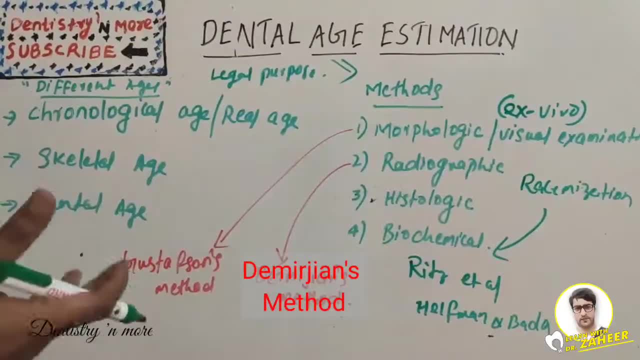 So various radiographic images that can be used in age identification are IOPAs, lateral oblique radiographs, cephalograms, the OPGs or digital imaging and any advanced imaging technology. Now let's focus on mainly the dermogeans method and Gustafsson method. 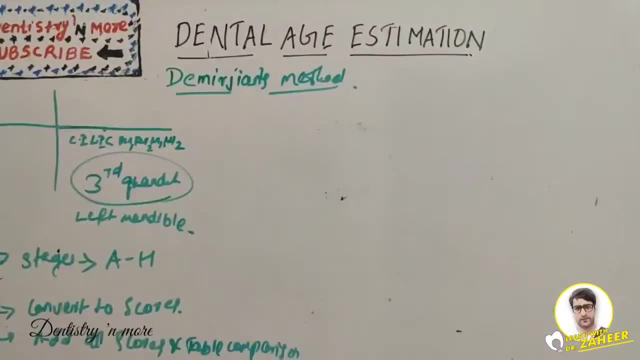 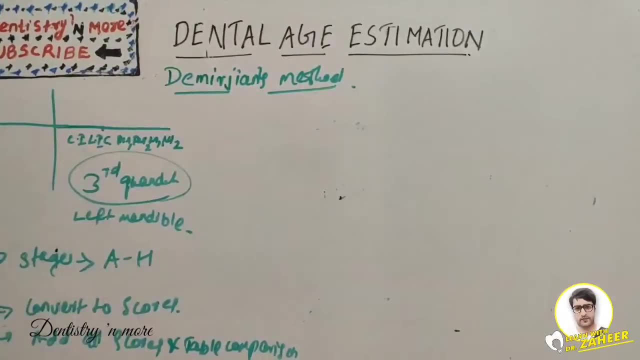 So in the radiographic method the most common one is the Demergeans method. So this Demergeans method actually started in 1973 by a group of people. So it uses the seven teeth In the left side of mandible, that is, the third quadrant teeth. 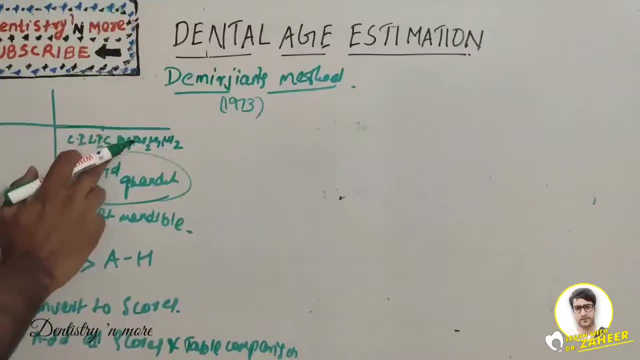 That is central incisor, lateral incisor, canine, first second premolar and first second molar. So this is the left side of mandible. That is the third quadrant teeth. Seven teeth are used And they used stages A to H. 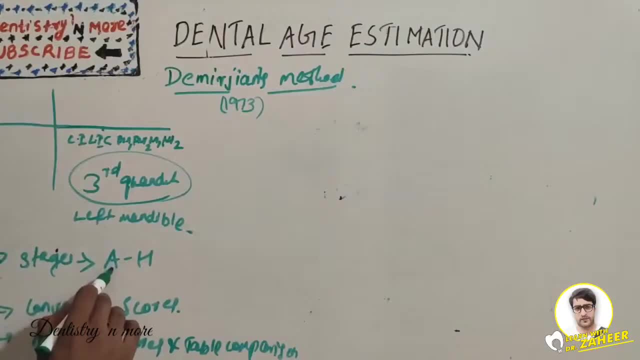 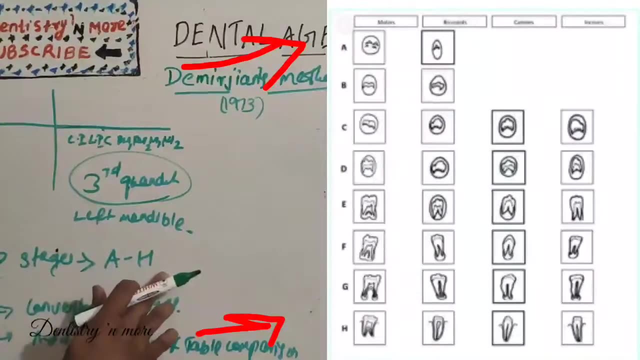 That is a stage which is having a minimal calcification- Calcification or tooth formation- and to the last stage. So these stages were used to mark the developmental stage of the tooth in the suspect. That is, the stages were formulated by Demergeans. 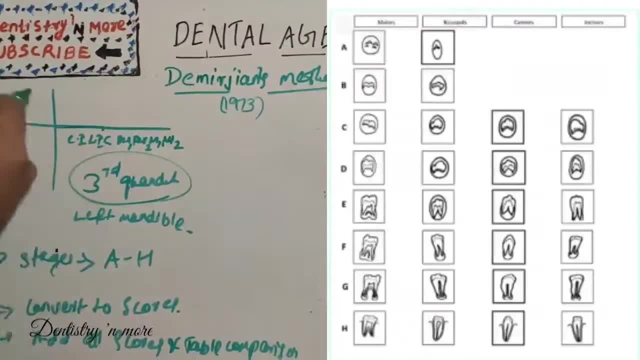 Which has usually marked by recognizable tooth shapes from the beginning of calcification through to final mature form. So these stages must be easily recognizable And such that a tooth always passes through the same stage in every individual So it can be easily correlated and calculated. 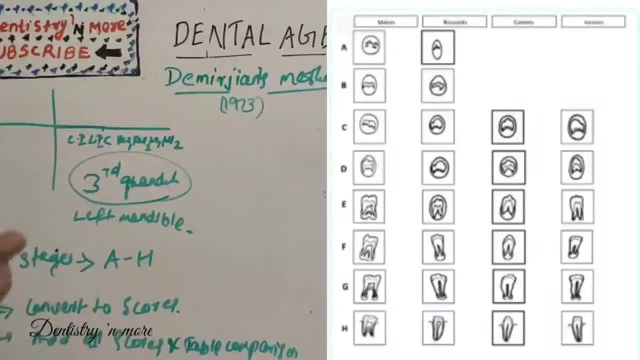 So since these stages are indicators of maturity and not of the size, They cannot be defined by any absolute length measurement. So We first select the seven teeth, So we start from the second molar, then first molar, second, first premolar, canine lateral incisor and central incisor. 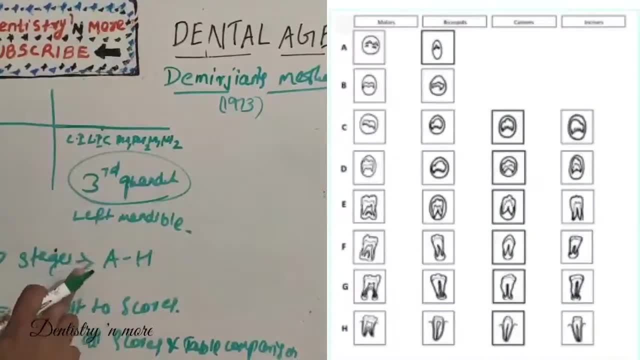 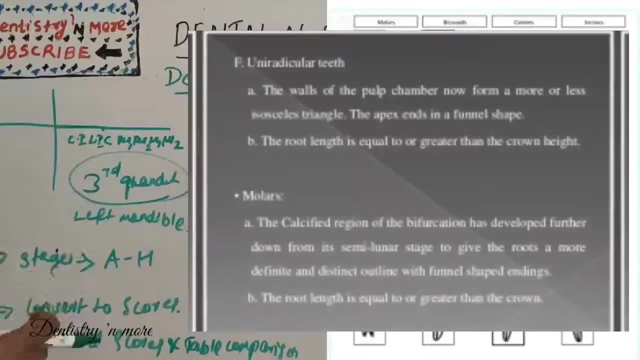 And all the teeth, all the seven teeth, are rated on a scale A to H, So the rating is assigned by following carefully the written criteria for each stage And by comparing the tooth With the diagram and X-ray pictures given for comparison. And for each stage there are one, two or three written criteria, which is marked by A, B and C. 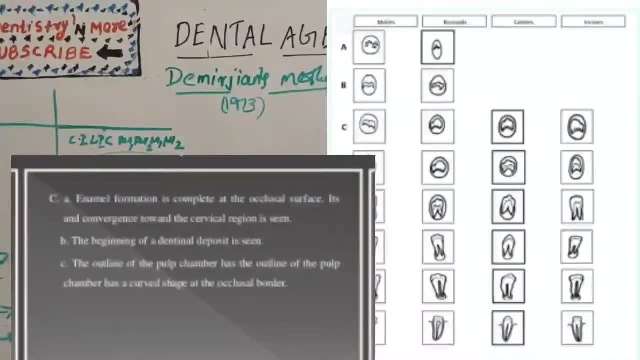 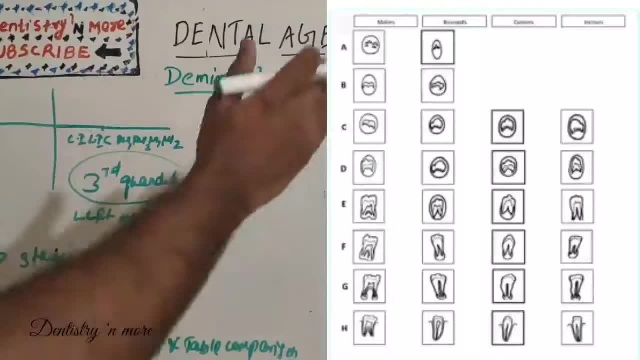 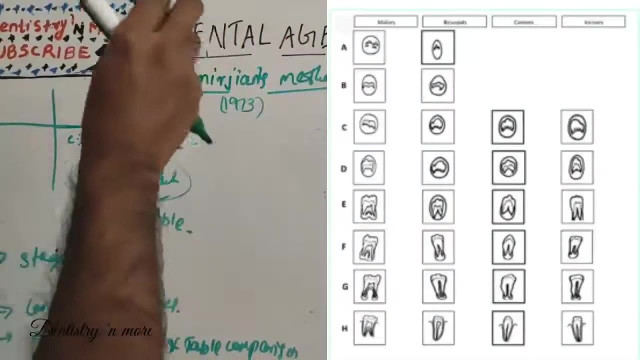 So you can see here the stages of Dermagen, That is, A to H, and its characteristics. So the stage A, That means you can see the picture here. It is a calcification. It is a calcification of single occlusal points without fusion of different calcification. 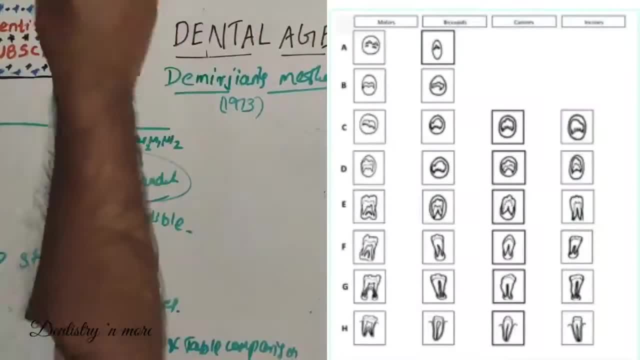 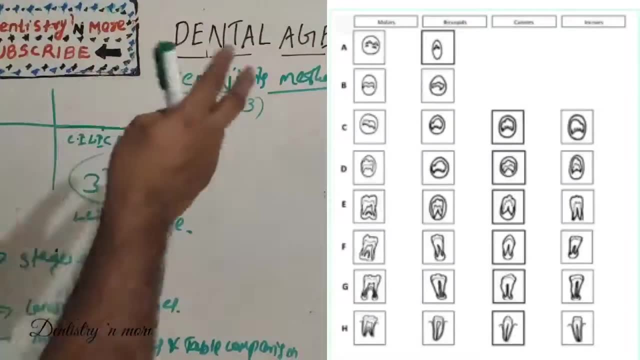 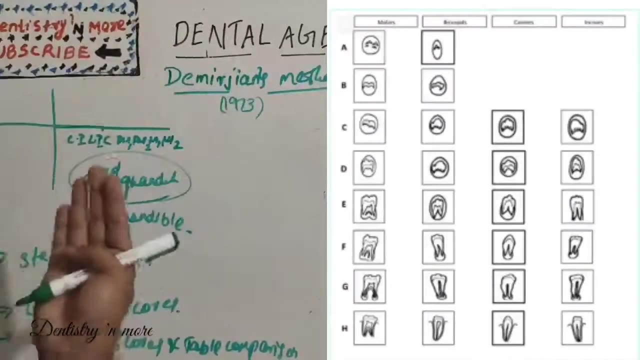 So we are going to compare it with our tooth And whether it matches the stage A or not, Whereas the stage B- fusion of mineralization points, the contour of occlusal surface is recognizable. So we compare the X-ray film of that particular mandibular third quadrant teeth with these images. 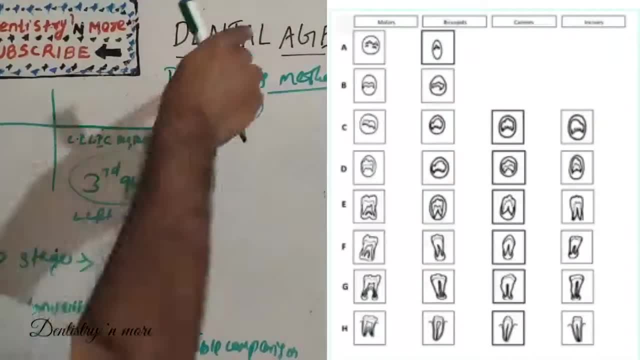 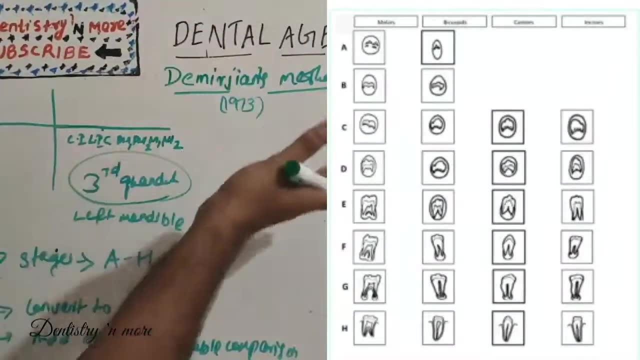 And find out where exactly our tooth matches. So, stage A, stage B, Stage B has occlusal surface recognizable, Whereas stage C is much more formation has happened: Enamel formation completed at occlusal surface And tentane formation has started. 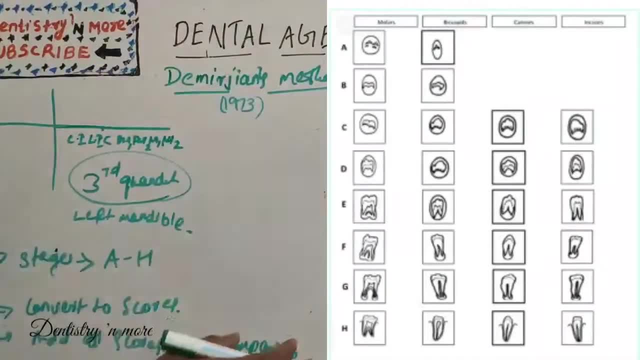 Pulp chamber is curved and now pulp haunts. So that is stage C. So we need to match it with our X-ray for each tooth. Then stage D: Crown formation completed at till the level of CJ, Root formation started, Pulp haunts are started. 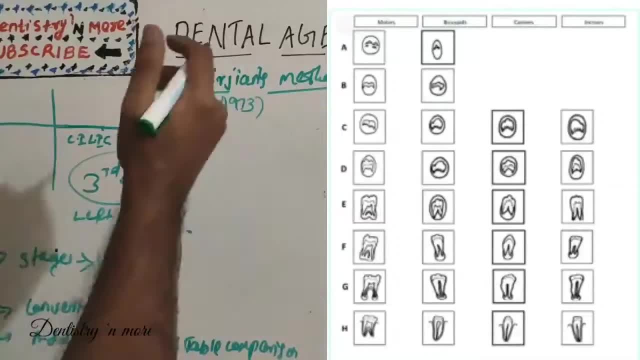 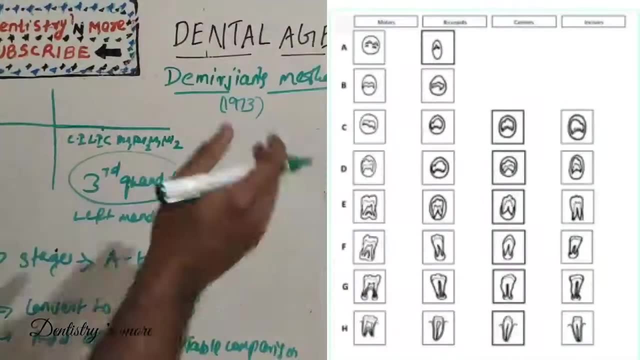 But the walls of pulp chamber remain curved. Whereas the stage E, The root length remains shorter than the crown height. The walls of pulp chamber are straight And the pulp haunts have become more differentiated than in the previous stage, Whereas the stage F. 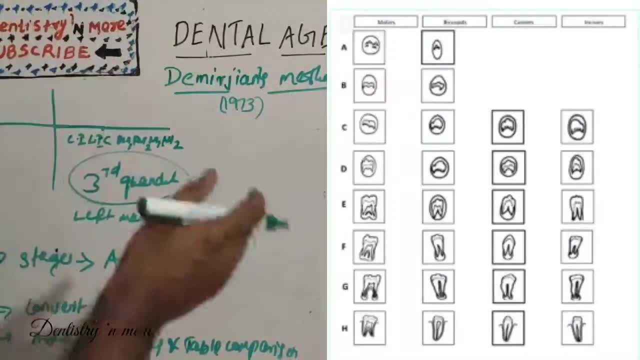 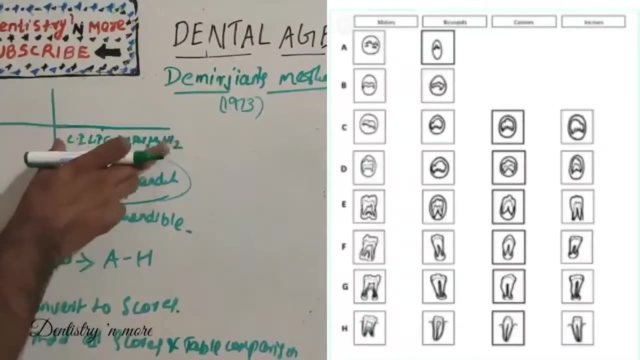 The walls of pulp chambers now form a triangle And the root length is equal to or greater than the crown height. In molars the bifurcation has developed sufficiently to give the root a distinct form. So we are comparing the X-rays of our particular patient's third quadrant teeth. 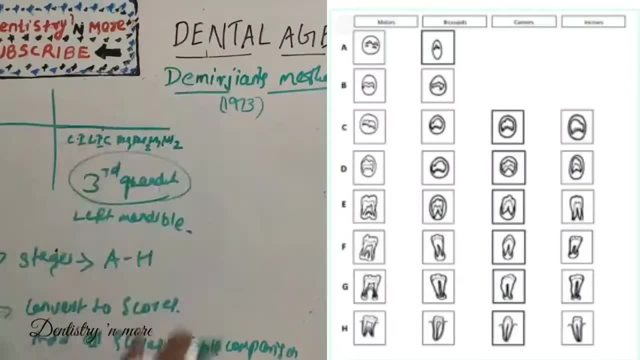 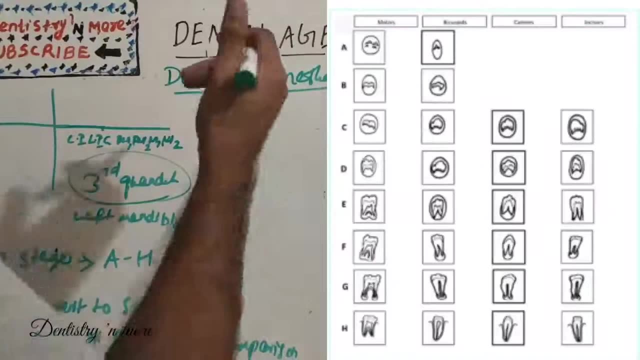 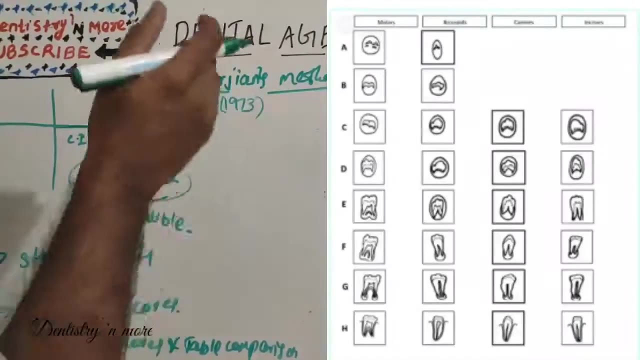 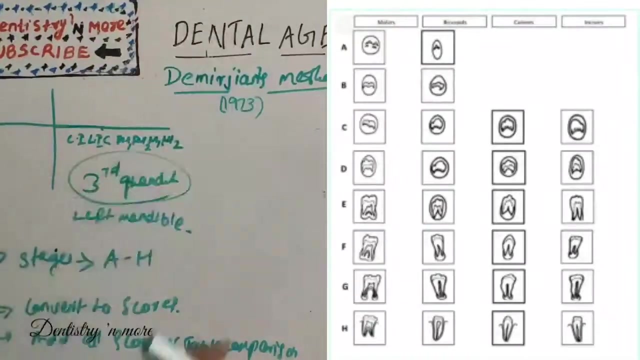 With this, dermagens A to H stages And finally we have G and H stages. In G stage the walls of the root canal are now parallel, The apical end is open And H the root apex is completely closed. The periodontal membrane surrounding the root and apex is uniform and width throughout. 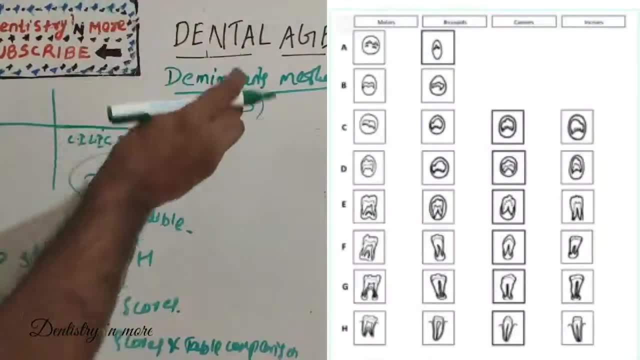 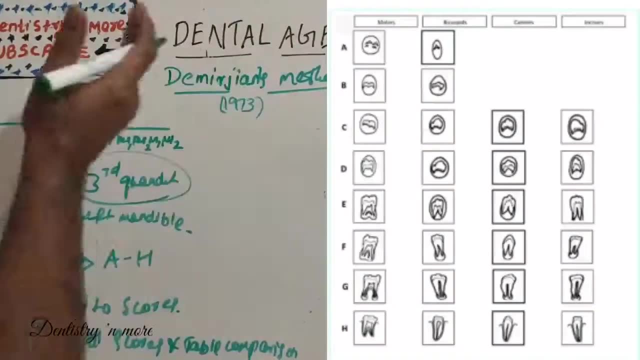 So A is the beginning of calcification and tooth formation, H is the completion. So we need to compare A to H stages with our tooth. Okay, So I told you. for every stage we may have one tooth.